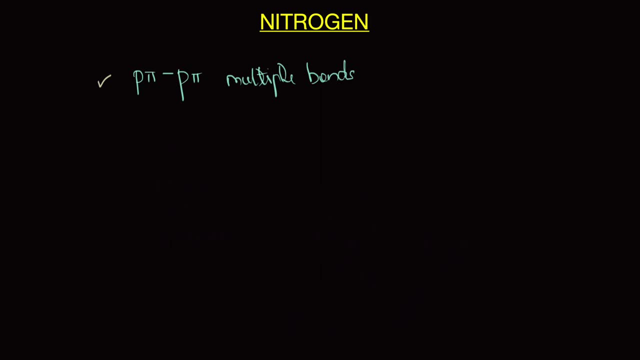 its chemistry. You see, just like Carbon of group 14, Nitrogen has the unique ability to form p-pi-p-pi bonds with itself and with elements that are similar in size and have high electronegativity, like Carbon and Oxygen. 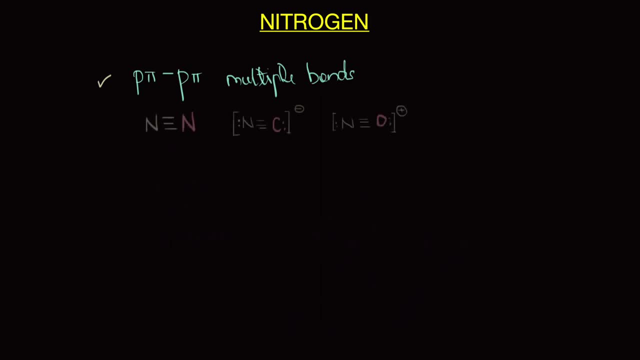 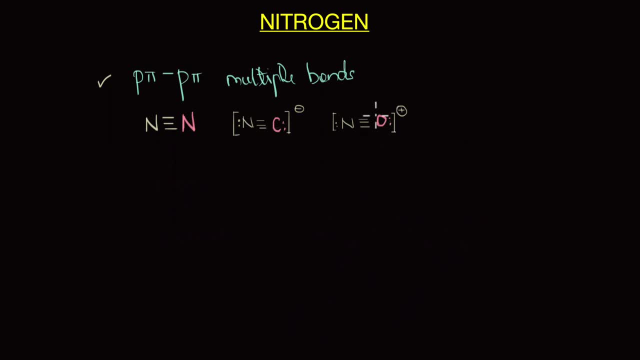 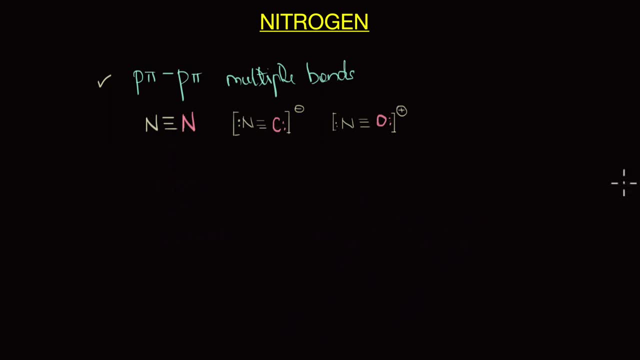 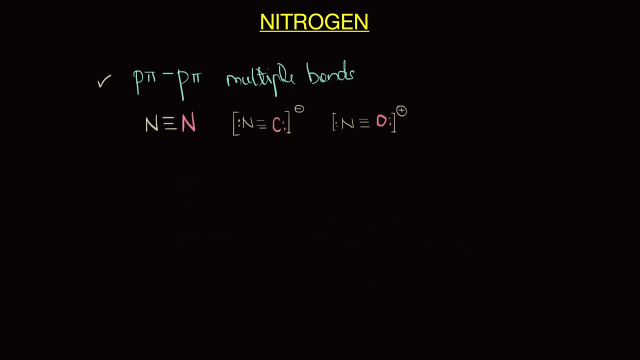 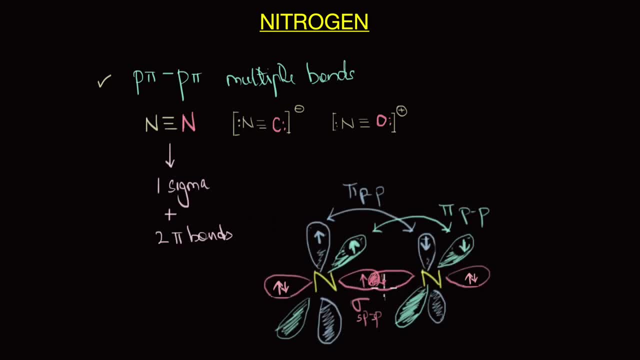 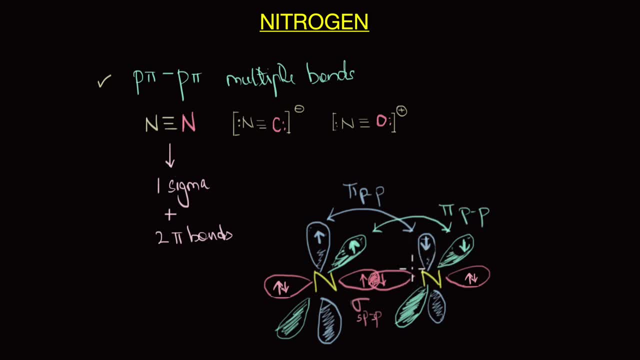 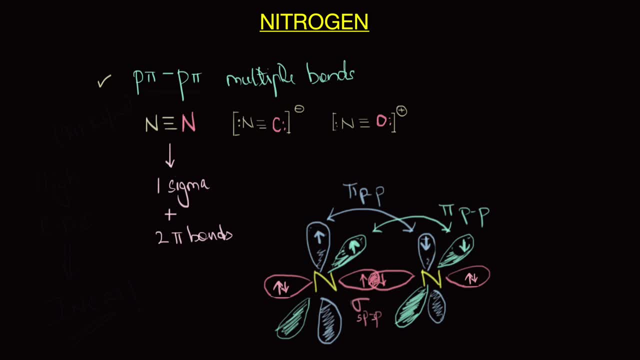 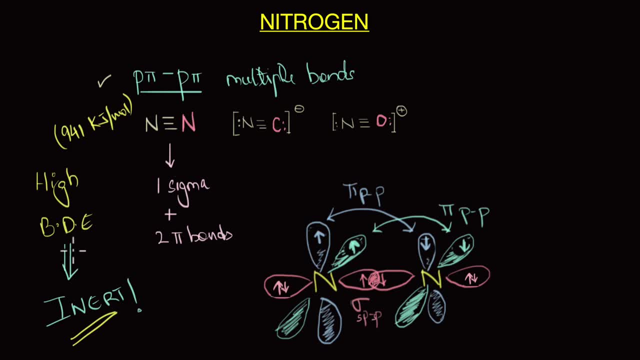 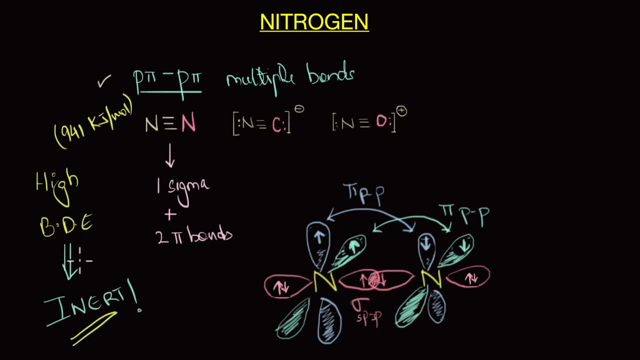 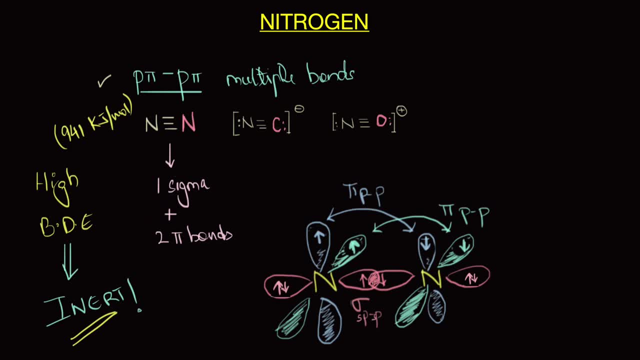 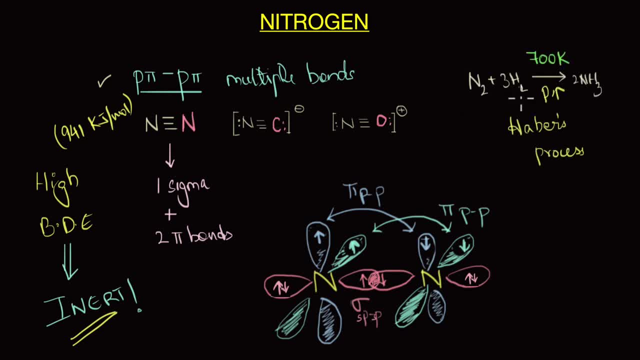 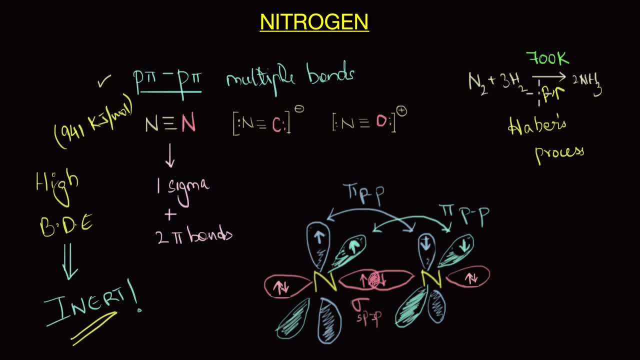 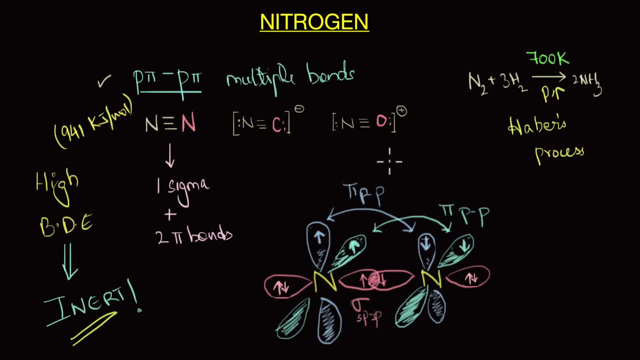 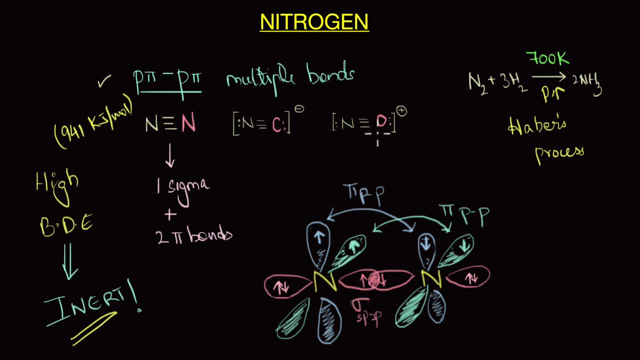